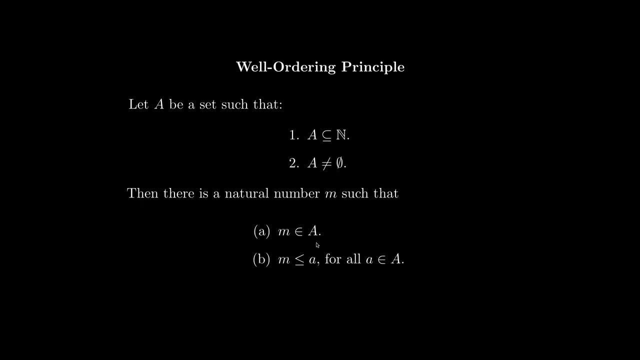 So the following happens: That natural number is in the set A and is less than or equal To any element of the set A. So basically, what we are saying is it has a minimum, and one important part here is that the minimum has to be in the set A. 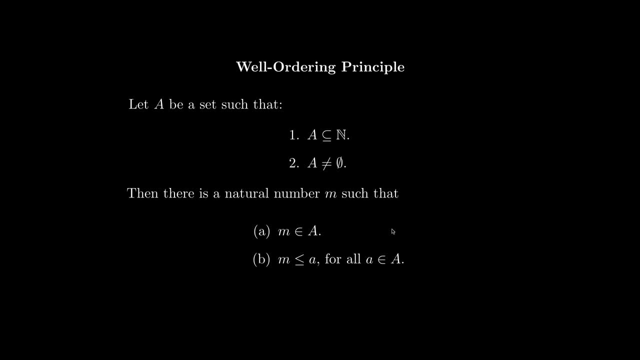 So that's an important part and is less than or equal to all the elements in A. So those two things makes a minimum is not enough. that is less than all the elements in A. It has to be in the set A. Now let's look at some examples and see how. 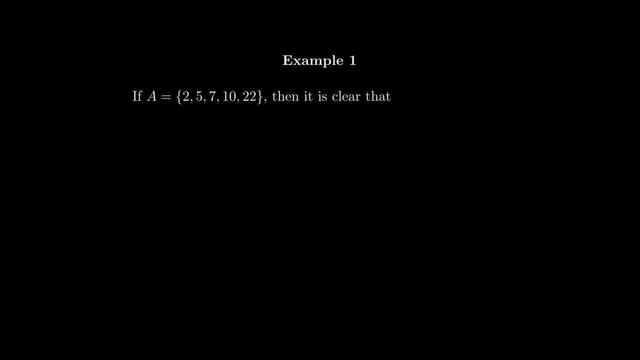 How this actually will work. So let's start with something very simple. Example number one: So let's say we take a set, that is, this collection of natural numbers- two, five, seven, ten, twenty-two- Then in this case, of course, that is a subset of the natural numbers and is non-empty, but it has five natural numbers. 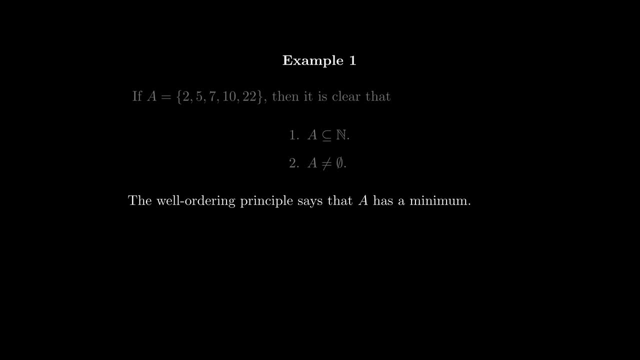 So the well-ordered principle says that A has a minimum, And the minimum in this case is, of course, two. Of course, this is a very simple example. You don't actually have to apply the well-ordered principle to see that A has a minimum, because A is quite simple. 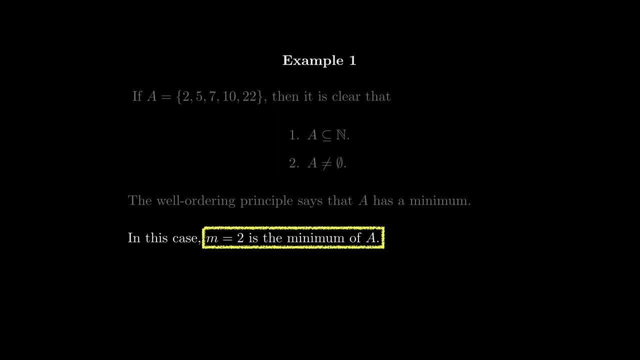 It's just a list of five numbers, So it's just very simple to see. As you can see there, just the number two is just the minimum of the set A. Now let's look at an example a little bit more complicated. So let's say we take 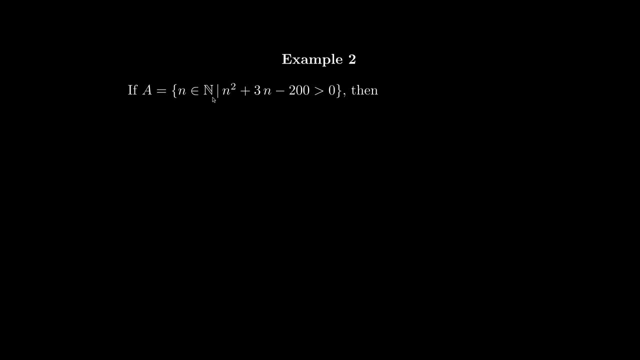 A set A, which is the collection of all the natural numbers that satisfy this inequality here, And the inequality is the square of the number plus three times the number minus two hundred is bigger than zero. Now, if we want to apply the well-ordered principle, we need to check some things first. 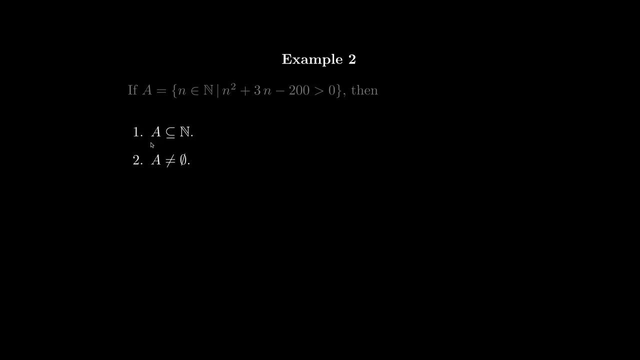 So the first thing we need to check is that the set A is actually included in the natural numbers And the second that is not empty. Now how do we know that is included in natural numbers? It is clear. That's because the definition of A says A is the collection of all natural numbers. 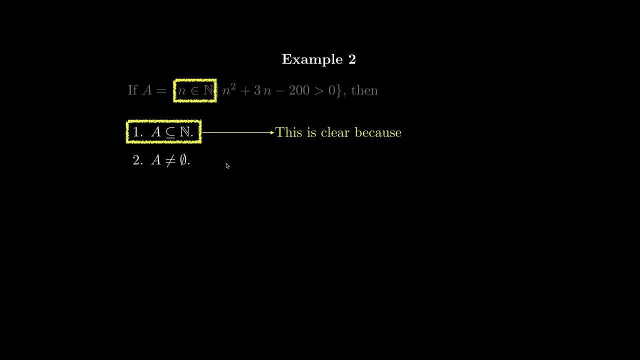 So, by definition, the set A is included in N. Now, the second condition that you also have to check- and that's also very important- is that the set is not empty. Now that is not clear. It's not as clear as checking number one. 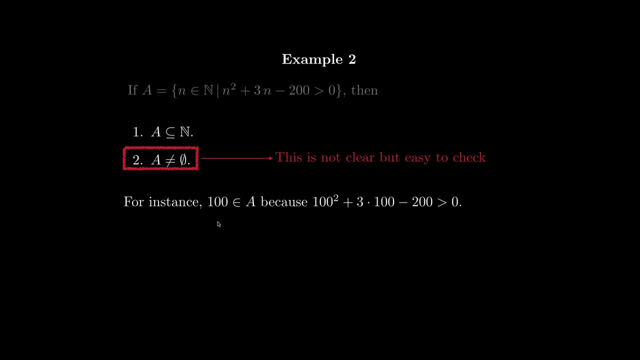 But is easy to check. So, for example, you can say: you can check that one hundred is in A. Why? Because one hundred is a natural number And it satisfies this inequality. If you just plug it in here, replace the N by one hundred, it will just be bigger than zero. 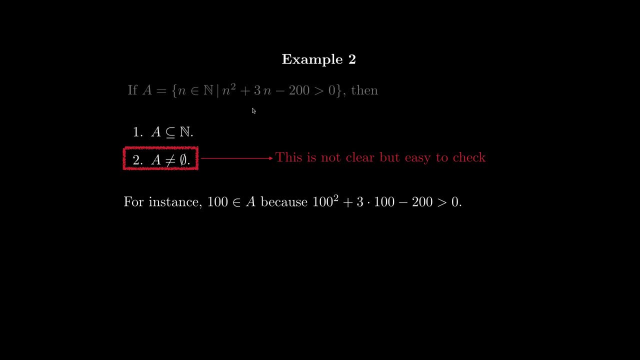 Now you can check with another number. Now it's not clear, but it's easy to check, Because if you can think about this inequality, you have to make it bigger than zero. So if you choose a large number, you probably will get this bigger than zero. 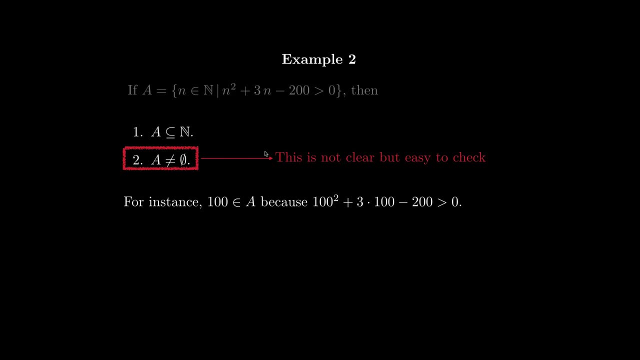 One hundred is just an example, but one thousand will work, or two thousand and so on, So we can check that it's not empty. So that is true. So we have the two conditions. By the well-ordered principle, the set A has a minimum. 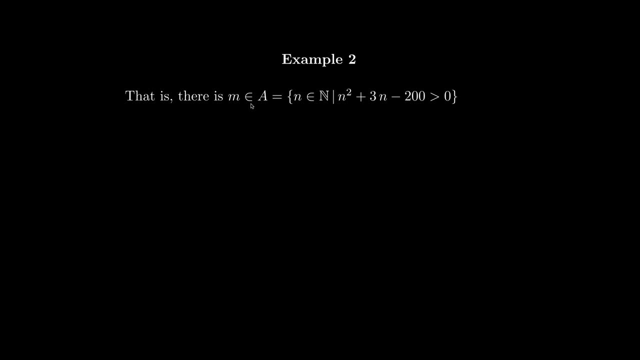 So that means that there is an element in this set in the collection of all natural numbers that is not empty. So that means that there is an element in this set in the collection of all natural numbers that satisfies this inequality, that is less than or equal to all the numbers, that satisfies that inequality. 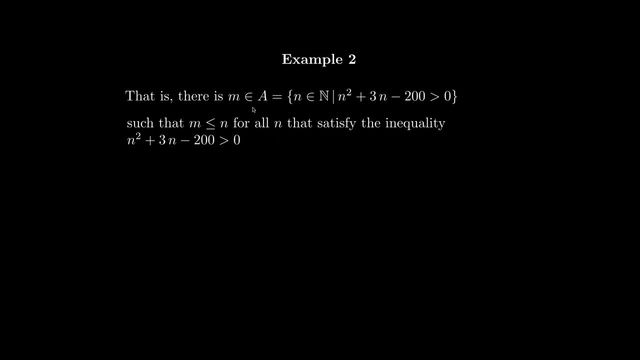 So there is an element in A that is less than or equal to everything else. Now, in this case we don't have the list of A, like we had in the previous example. We have a descriptive way of the set A, So it's described by this inequality. 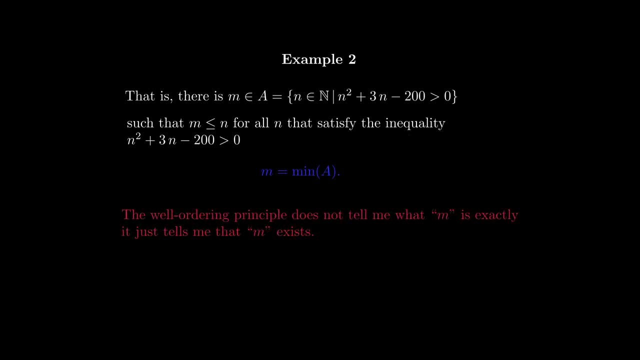 So we know that there is a minimum of the set A. Now, one thing that is important in the well-ordered principle is that the well-ordered principle does not tell me what M is exactly. It doesn't tell me how to compute it. 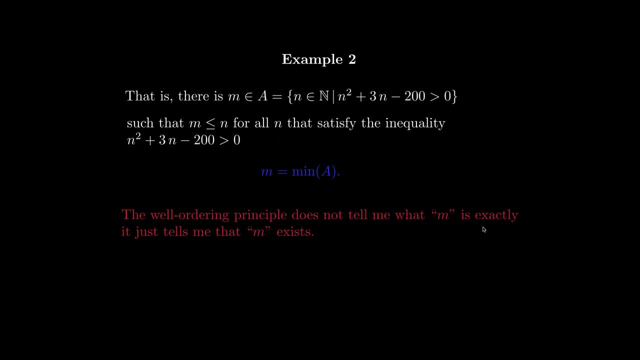 It just tells me that it exists. It has a minimum. Now computing the minimum, that's just another matter. The well-ordered principle is a principle about existence. It tells me that something exists, but it doesn't tell me what it is. 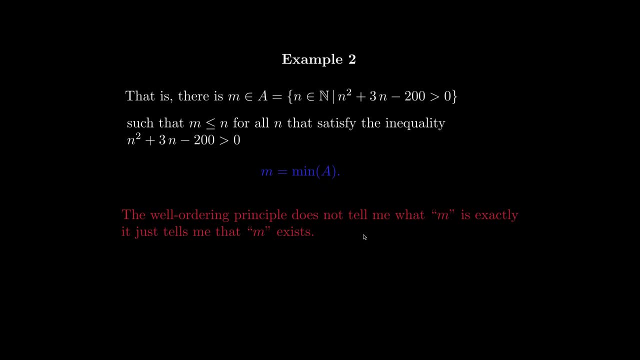 It just tells me how to compute it. That's just another matter completely. Now, in the example number two we had, which is this inequality, we can check that this, the collection of all natural numbers that satisfies this inequality, is 13,, 14,, 15, and so on. 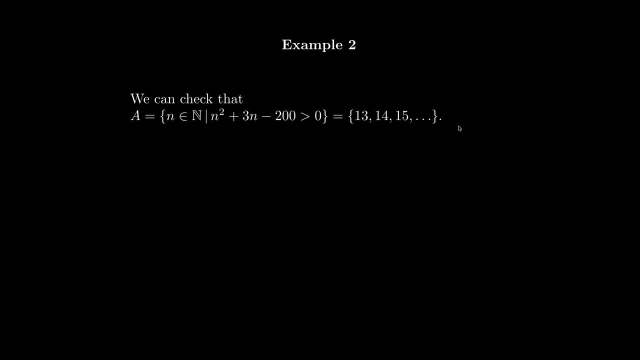 Now, that is not difficult to check, but it's not that clear either. Now, if you want to check this from the point of view of the graph of the inequality. so if you look at this expression here: n squared plus 3n minus 200,. 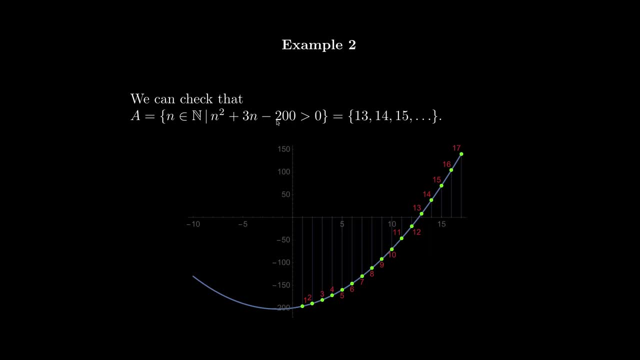 that is a quadratic equation. that will give you a parabola, which is this graph that you have here in blue. that is a parabola. What we're looking at is looking at the natural numbers. So when you plug it in here, it gives you bigger than zero. 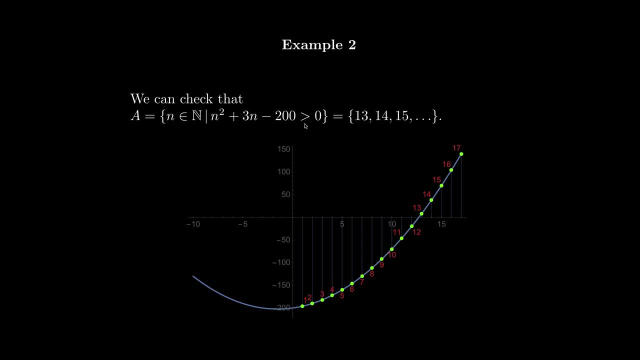 So we are looking at the natural numbers that make this bigger than zero, or, in terms of the graph, they will be above the x-axis. As you can see here, I labeled the points 1,, 2,, 3, 4 for the natural numbers on the x-axis. 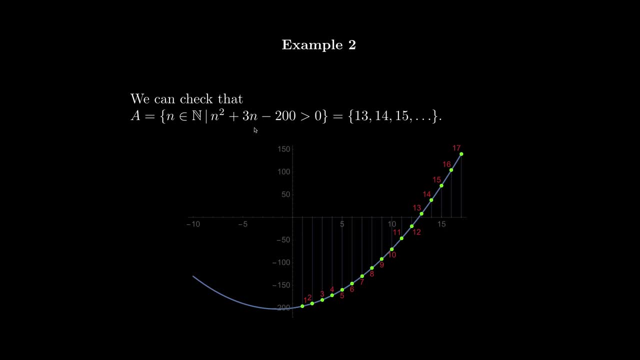 and the points that they correspond on the actual graph of this parabola. So, as you can see here, the points start to get over or above the x-axis after the number 13.. So 13,, 14,, 15,, 16, and 17,, and so on. 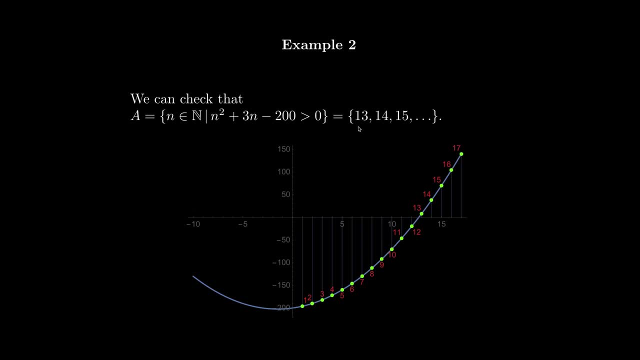 So this is set. A is an actual infinite set, And if you knew how to solve this inequality, then you will realize that 13 is the minimum. but that's not the point of the well-ordering principle. The well-ordering principle simply says that you have a minimum. 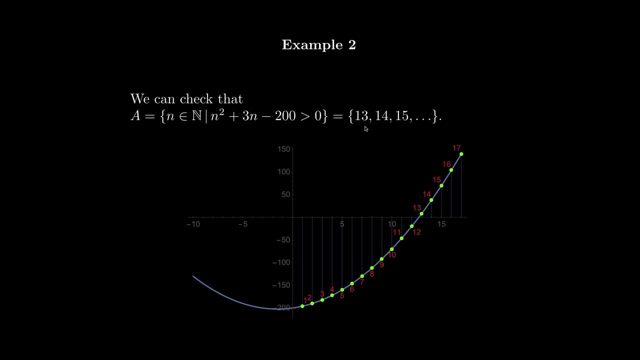 How you compute it. that's just something different. So let's look at this example, example number 3.. So let's say we have a set here and let's introduce some trigonometric functions for this example. So let's take the set A. 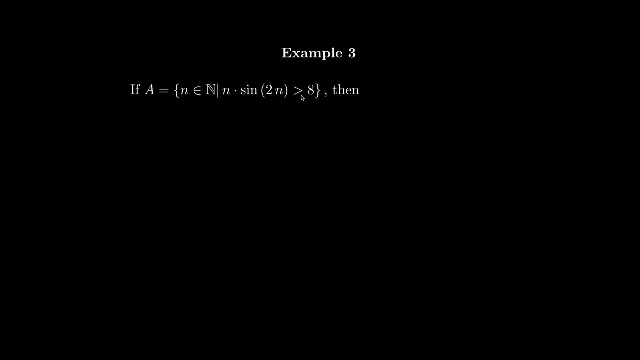 So for the natural numbers that satisfy this inequality here. so n, the number n times the sine of 2n is bigger than 8.. So we're going to look at natural numbers that satisfy this inequality here. Then, if we want to apply the well-ordering principle, 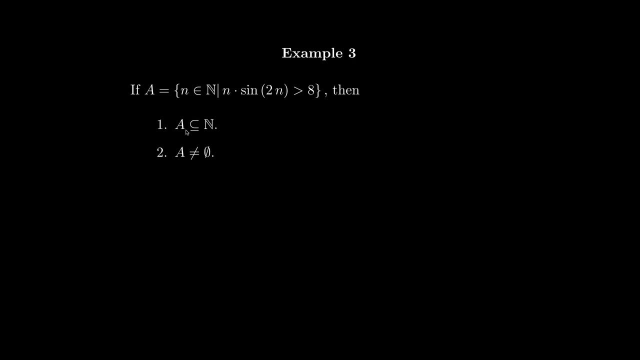 we need to check 1 and 2.. So we need to check that it's a subset of the natural numbers and we need to check that it's not empty. Now checking that it's a subset of the natural numbers. that is just clear from the definition of A. 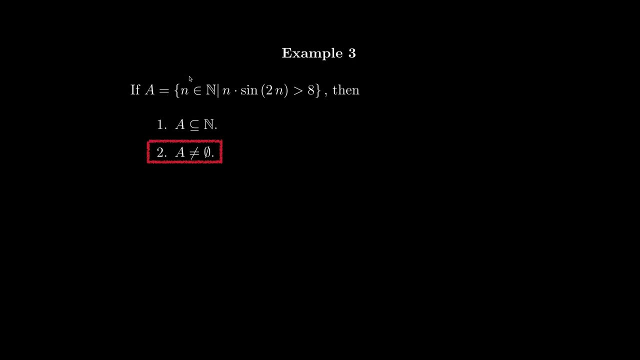 That's because this part here is what it tells me- that it's a subset of n of the natural numbers, Because it's by definition. you take all the natural numbers that satisfy this property. So by definition it is already a subset. 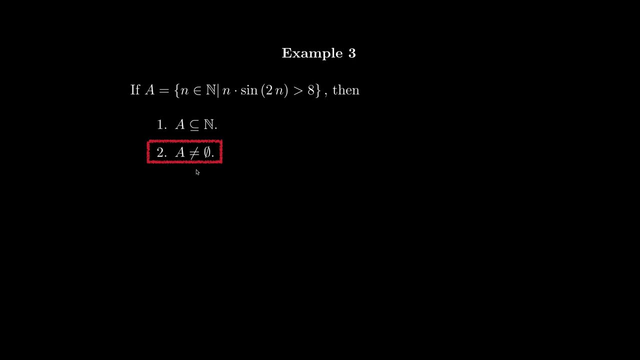 Now the second part, which is checking that it is non-empty. that is not difficult, but isn't clear either. Now, checking that it's non-empty means that you at least have to find a natural number that satisfies this property, Or a more complicated way to do it would be to solve the inequality. 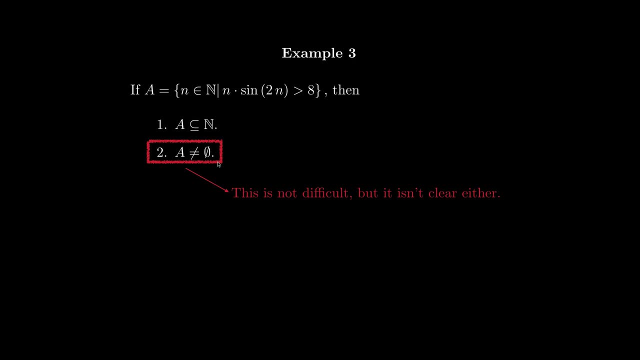 But to check that it's non-empty, you only have to find one, One natural number that satisfies this property. So that's all you need, And so that's why I say it's not difficult, but it's not clear either. So we can numerically check that 13 is in A. 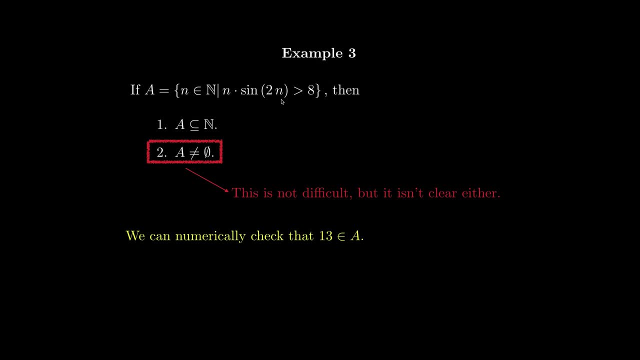 So if you plug in 13 here, then you do this computation here on your left and that's going to give you bigger than 8.. Now when you do this and you plan to do this with your calculator, so make sure that it's in radians, not in degrees. 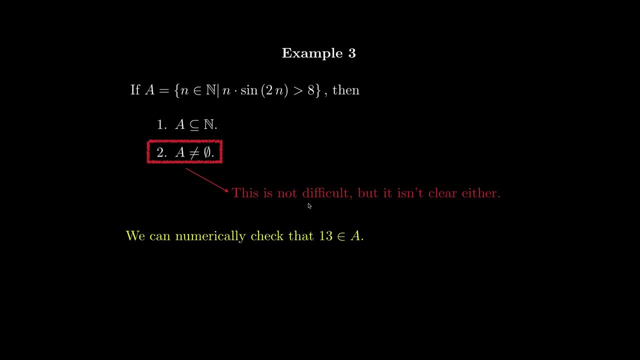 So if we check that 13 is in there using your calculator or some other method, you can see that it's bigger than 8, so that set will have a minimum value, And it will have a minimum because it's a subset of natural numbers. 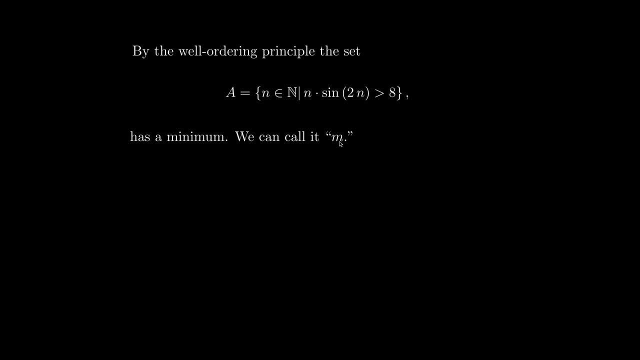 it's not empty. So we call that minimum, we call it M Again. what the where order in principle says is that it has a minimum, but it doesn't tell me how to compute it. That's the whole point. Now, it's not trivial to see that the actual set A. 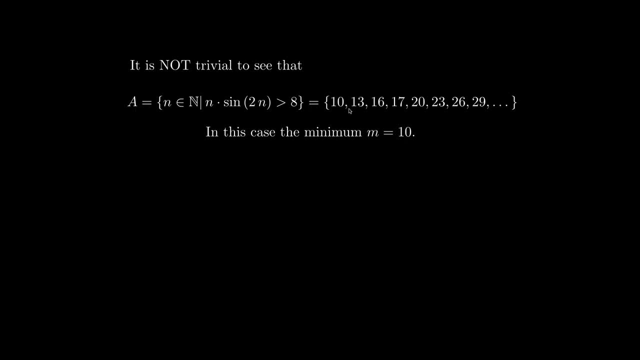 which is defined here by this property is actually this collection of numbers: 10,, 13,, 16,, 17, and so on. Now, to realize that this is equal to this one, you will actually have to go ahead and solve the inequality. 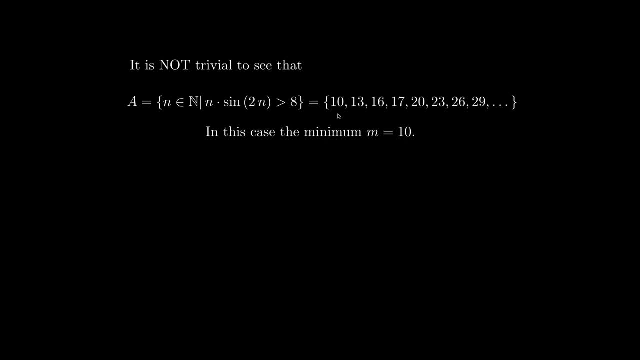 So in this case, if you believe that this solution is correct, then the minimum will be 10.. But that's not the point of the where order in principle. The where order in principle doesn't tell me that it's 10.. It's just that by some other method. 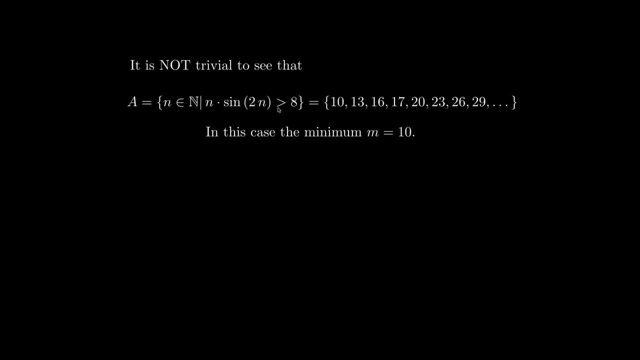 we know that this is the solution of this inequality, This inequality for natural numbers. So in this case, the minimum is 10.. And if you want to look at this graphically, if you look at this graph of n sine of 2n, 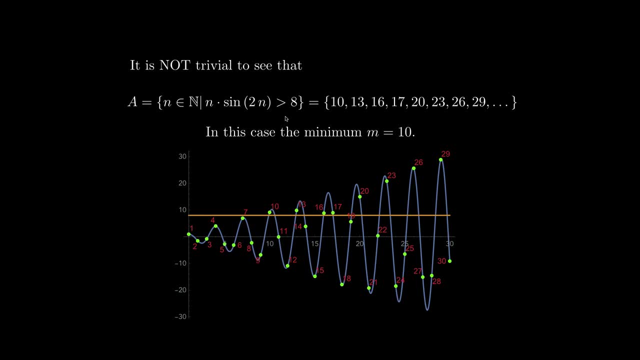 I have that graph here in blue And we are looking to see when is that bigger than 8.. 8 here will be represented by this horizontal line that is in orange here, And so we're looking at the natural numbers that make that bigger than 8,. 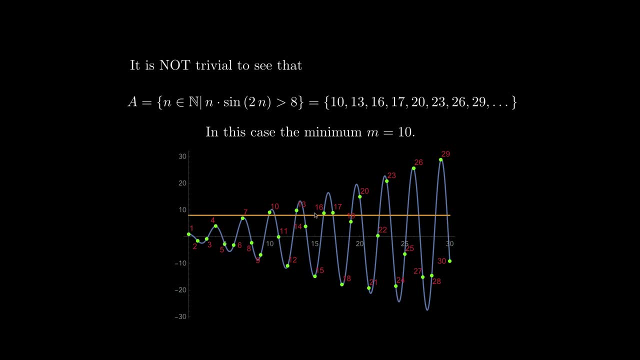 above this line here. As you can see, here some numbers are above and some others are below. So for example, the stars above that line at 10, but at 11 is less than 8, and at 12 is less than 8,. 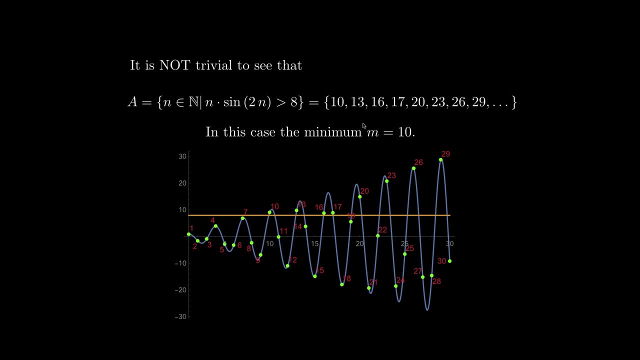 and it comes up again at 13- is bigger than 8.. That's why you have 10,, 13,, 16,, 17, and so on here. So this really is not a consecutive collection of natural numbers. It just goes up and down. 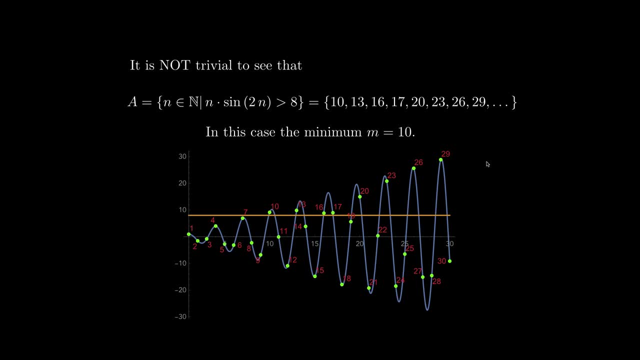 Because of the nature of this trigonometric function here. But again, this is not part of the actual well-ordering principle. This is just an example. The well-ordering principle only says that it exists, but it doesn't tell me how to compute it. 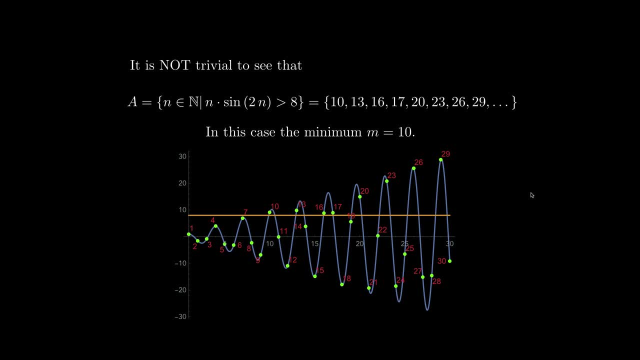 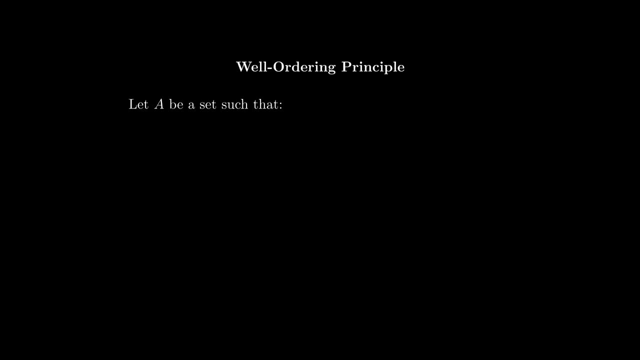 So this, what I'm showing you here, is just a way to visualize what is actually happening with this particular example. Now let's just review again what the well-ordering principle is. So you have a set A that has two properties. 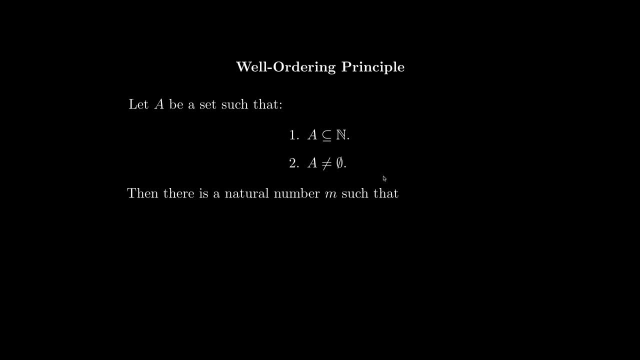 that is a subset of the natural numbers and is not empty. So there is a natural number, m, so that is the minimum. So it's in A and it's less than or equal to all the elements in A. Important that the minimum has to be in A. 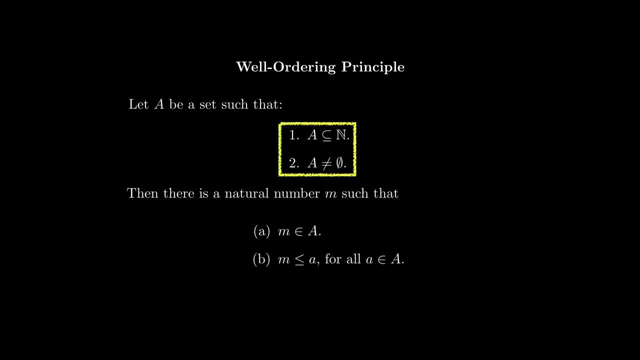 So that's an important part. So those two properties you always have to check. so there's conditions to be checked and once you check that then you can make the conclusion. Now, as I mentioned earlier in the video, checking that the set is non-empty is important. 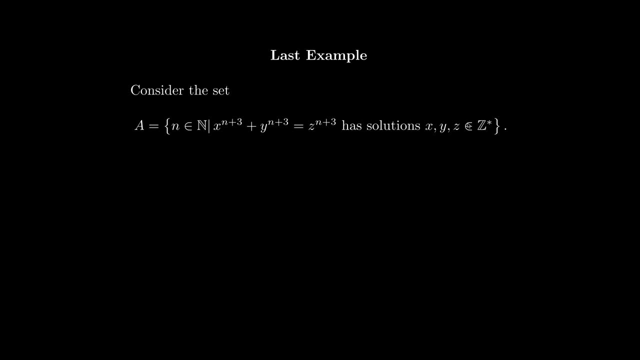 So let's look at this last example here. So if you look at the collection of all the natural numbers, n, so that this equality here has solutions x, y and z for the integers that are non-zero. So basically, what I'm looking at here is: 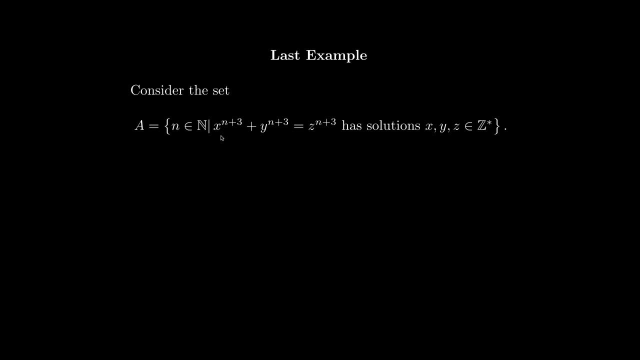 I have this equation and I'm looking at all the natural numbers for which this equation will have solutions in the integers. Now, this set here is clearly a subset of the natural numbers. Now the question is: can I apply the well-ordering principle? 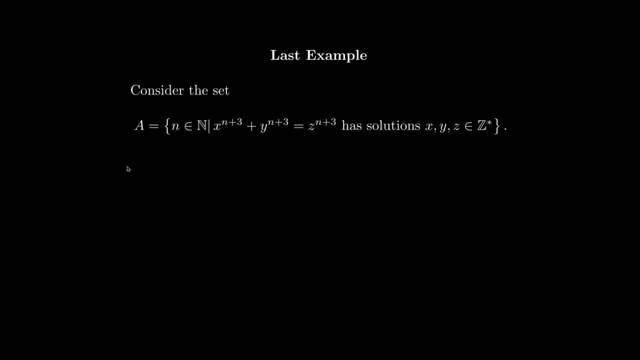 Well, you could, if you could prove that this set is not empty, But unfortunately that set is empty. So what that means is, if you look at this equality that is here, there are no solutions in the non-zero integers, And that is actually a very famous theorem. 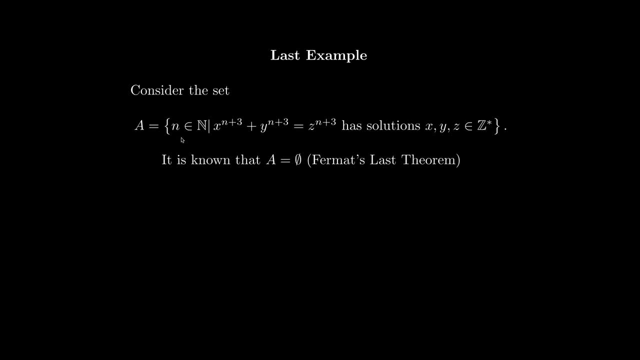 called the Fermat's Last Theorem. So even though, then, this is a subset of the natural numbers, you cannot apply the well-ordering principle because the set is just empty. So it doesn't make sense to talk about a minimum in A, because there is nothing in A. 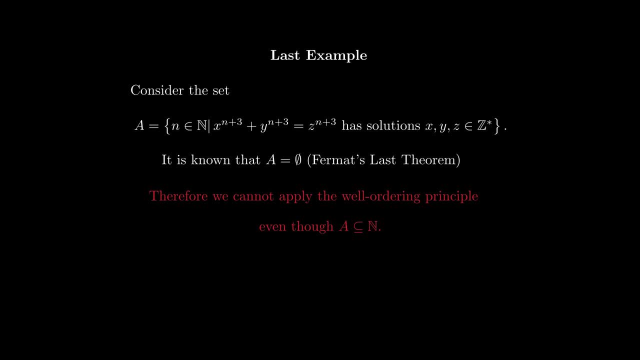 So, even though it's a subset of the natural numbers. Now, the well-ordering principle is not true when it's applied to other collection of numbers, like I mentioned before. So for the integers, rationals, real numbers and complex numbers, 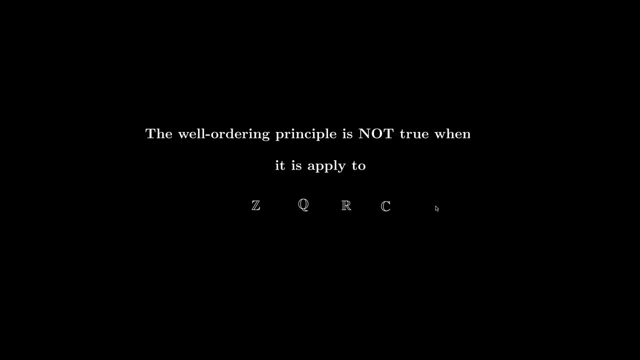 the well-ordering principle is not true. So what do I mean by that? Let me get into a little bit more detail about it. So the well-ordering principle is remember again. so you have these two conditions: one and two. 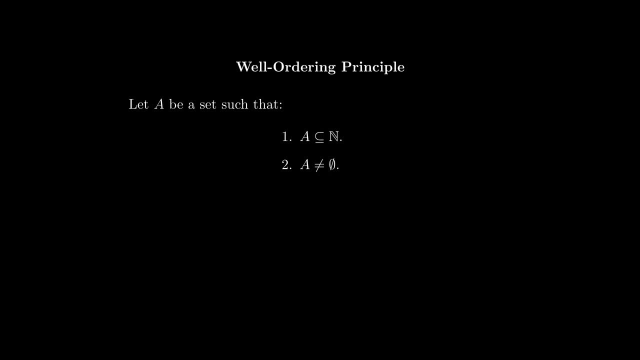 subset of the natural numbers non-empty. So the subset will have a minimum that we call m. Now let's assume that we replace the set n by the integers, for example, So we change it into an integer, And then can we make the conclusion. 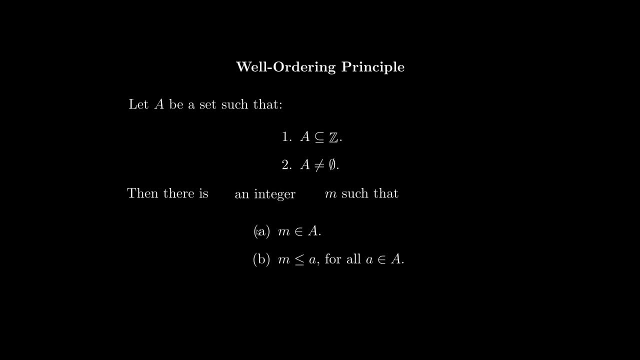 that there is an integer for which this is true. So the answer to that is that this statement, as it is right now, is not true in all the cases. So what does that mean? It means that you could have subsets of the integers. 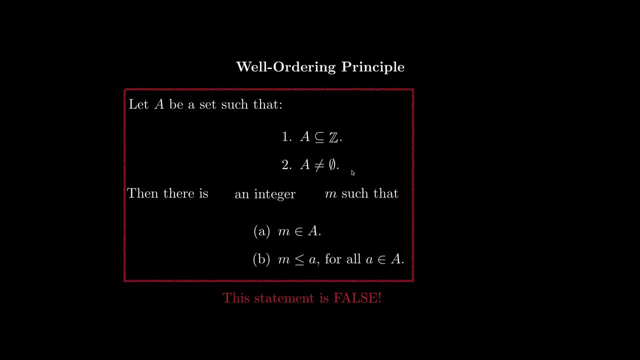 that are non-empty but that set won't have a minimum. So to prove that that is the case, I just have to give you some examples. This principle is not true in the integers. So let's look at some examples So we can have some non-empty. 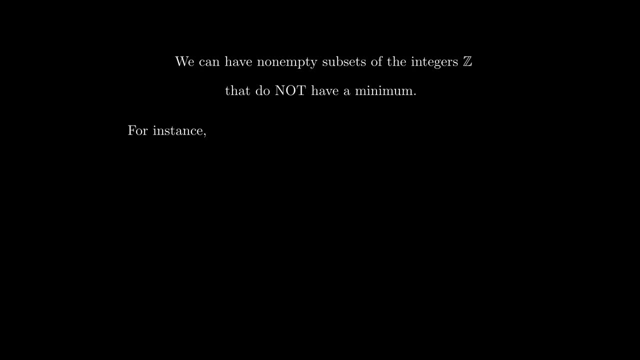 subset of the integers that don't have a minimum. So, for example, if you take the set a, that is the negative of all the natural numbers. so negative one, negative two, negative three and so on, that is a subset of the integers. that's true. 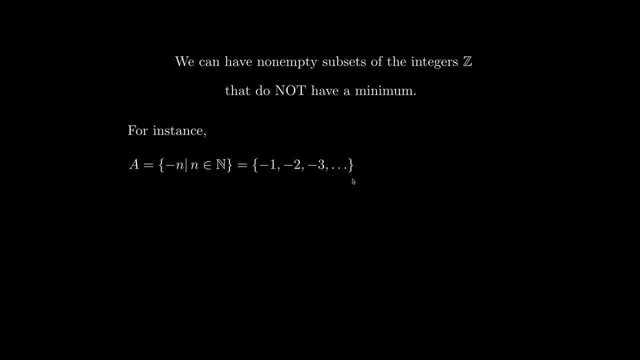 and it's non-empty. of course, it's true, but this set, as you can see, won't have a minimum, because the numbers just start getting smaller, smaller in the sense that, okay, is negative three the minimum? No, because negative four is less than negative three. 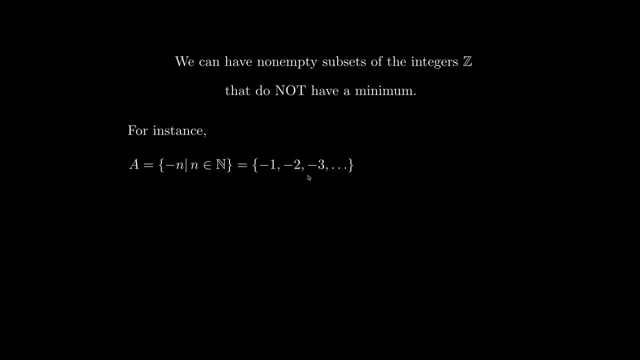 negative five is less than all the previous ones, and so on. So this set won't have a minimum And there are many examples. So if you consider, for example, the negative of all the squares of the natural numbers, so negative one, negative four, negative nine, and so on. 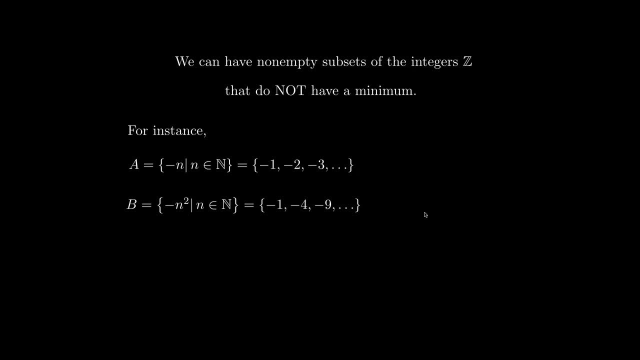 that is, a subset of the integers, is non-empty, but it doesn't have a minimum either, And you can come up with several examples, probably. so all the even ones negative, even ones negative, two negative, four negative six. 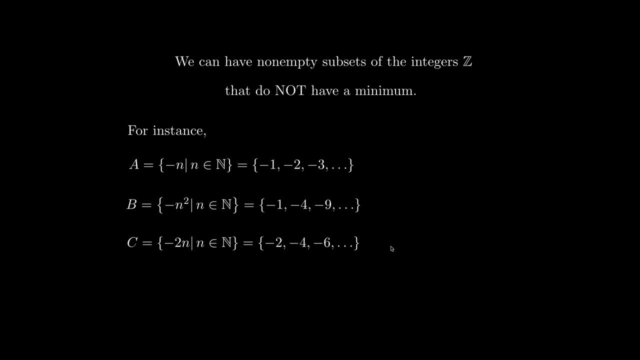 that is again a subset of the integers, is non-empty, but it doesn't have a minimum And a similar argument. you can make it for the rationals and the real numbers. so you have. you can probably come up with examples of subsets of rational numbers. 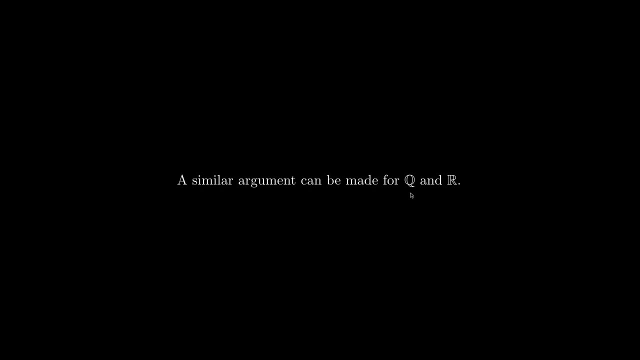 that are non-empty, but they won't have a minimum, And the similar thing for the real numbers. So the well-ordering principle is not true in the integers, in the rational numbers or the real numbers. Now for the complex numbers. 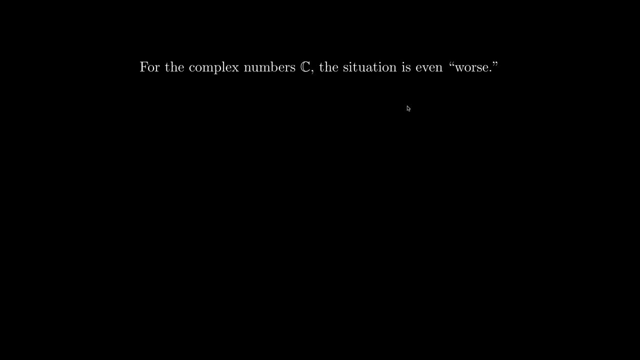 the situation is even worse, and the reason for that is because I'm going to explain why Now. so even though you can introduce some ordering in C? um, so like lexicographic, anti-lexicographic, and all of that, 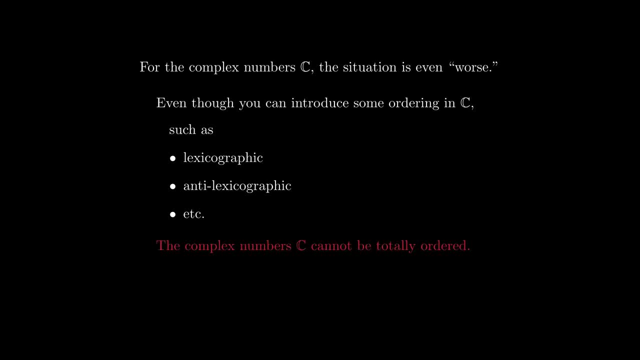 you cannot talk: uh, the complex numbers cannot be totally ordered. Now, if this is a little bit confusing for you, basically what this means is: um, you cannot order the complex numbers in a sensible way, Because if you want to have a minimum, 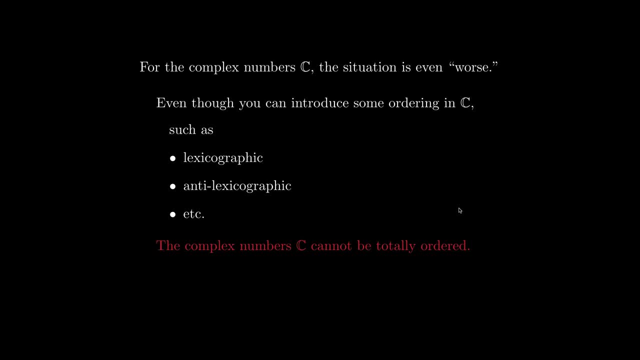 that means you can always compare two numbers and tell which one is the smaller one. In the case of the complex numbers, it is not possible to have a sensible way to always compare two- uh, complex numbers. that is totally ordered. So 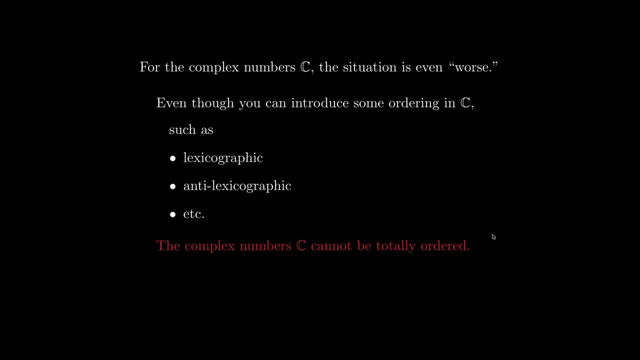 having a minimum will make sense. So even for the, so for the complex numbers, having a minimum will not even make sense, Even if you come up with some type of ordering for the complex numbers. So the situation is even worse for the complex numbers. 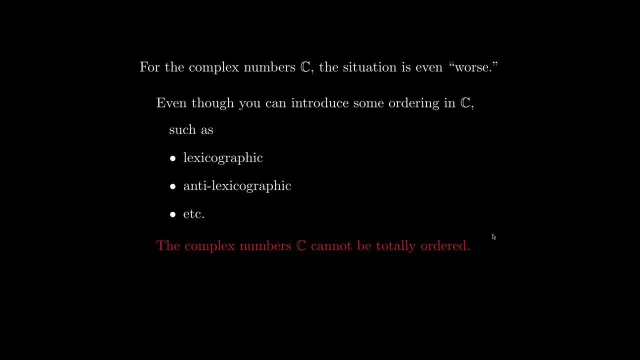 You cannot order Now the integers. the rational and the reals are thought, uh are ordered. You can introduce some order and maybe talk about minimums in some cases, but in the case of the complex numbers that that won't be. 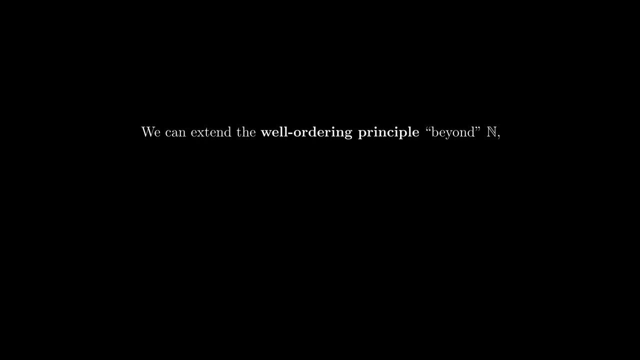 uh, possible. Now you can extend the well-ordering principle for subsets beyond n. So in in the set A, there are a lot of steps that I'm gonna explain. So you the only thing that you have to make sure, 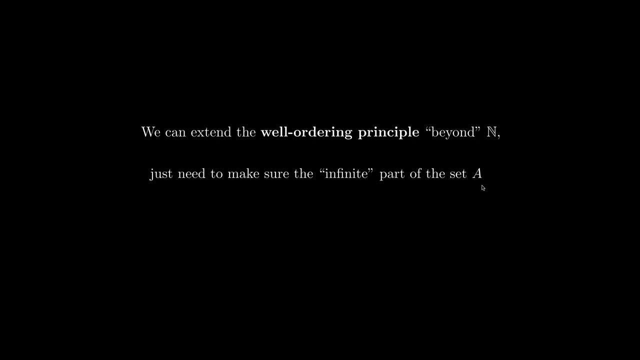 is that the infinite part of the set A is contained within the natural numbers, And I will explain this with a picture. So if you have the natural numbers, let's. let's imagine that the natural numbers is: ah, this diagram here. 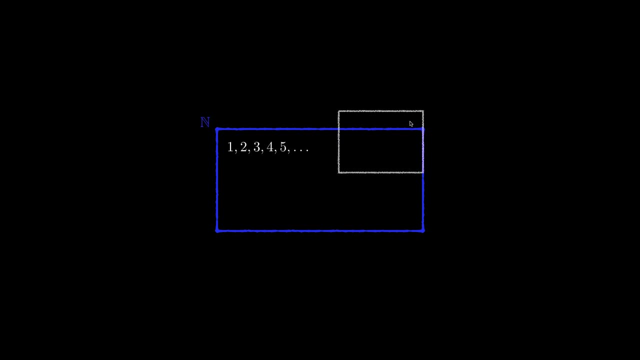 And let's say you have the set A and the set A is not completely containing n one. this will, this white square here, will be represented. my set a. it's not completely containing n. some part of it is outside, but the part that is infinite. 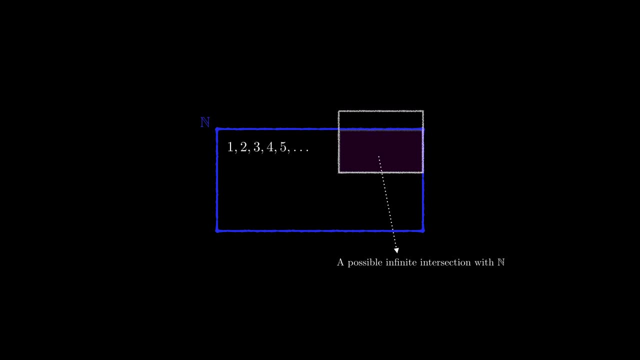 possibly infinite or potentially infinite, will be inside n, and the part that is outside n is is finite. if you have that, then the well ordering principle will also be true in this particular case, even though the set a is not completely containing n, and the reason for that is this: if you look at 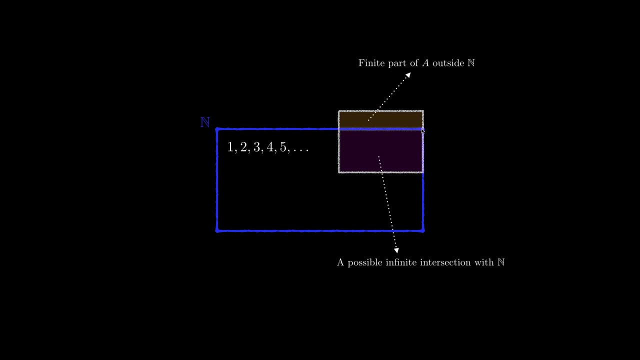 this setup but we have here. you can apply the well ordering principle to the part that is in inside n, so that will have a minimum here. and because the part outside n is finite, it will have a minimum as long as it's not empty. so any finite set has a minimum. 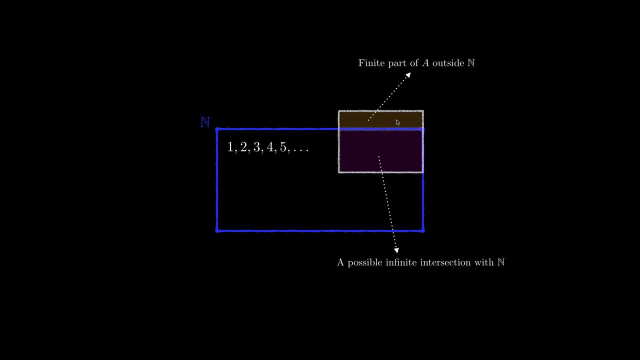 you don't have to apply the well ordering principle for that. the part that is important about the well ordering principle is: if you have an infinite set, then it will have a minimum. so this part here is going to be controlled by the natural number. so the infinite part of a is in. n will have a. 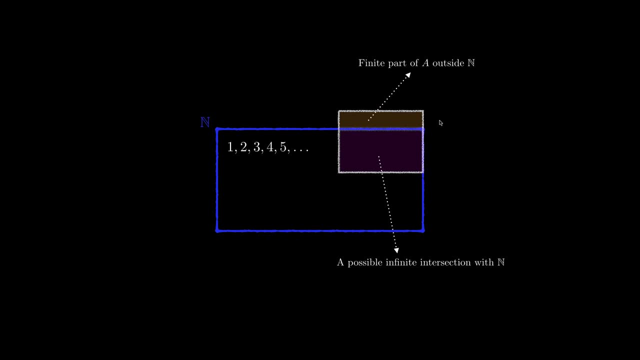 minimum and the part that outside, if it is finite, will have a minimum. so you compare the minimums of these two and choose the smaller one and that will be the minimum. so that's kind of an extension of the well ordering principle. now we might not use this in the class or the proofs or anything like that, but 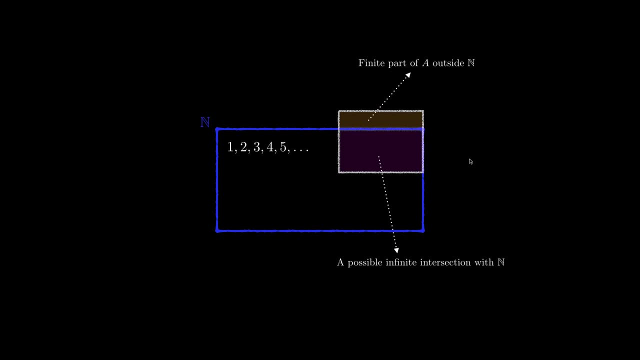 it's important to note that you can extend a little bit the well ordering principle, and that's all I have to say about the well ordering principle. we will continue with the lectures on number theory and I hope that this has been helpful for you. thank you for watching and I will see you next time.